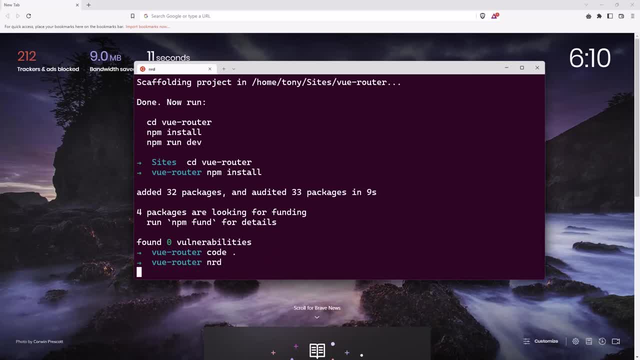 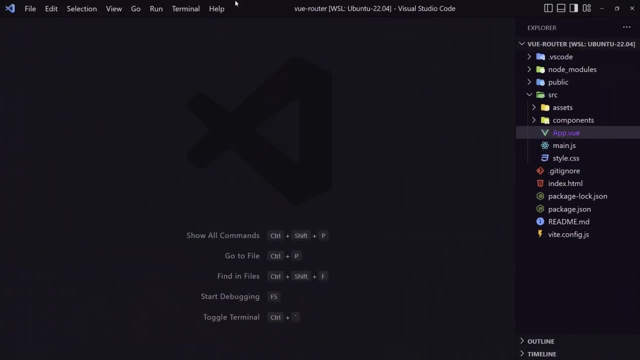 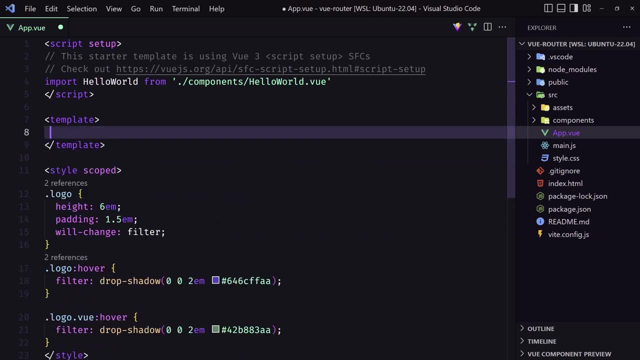 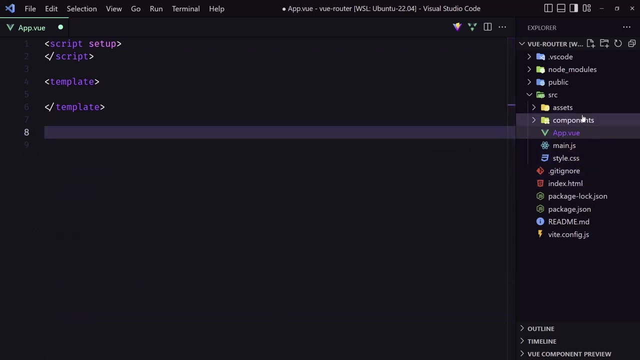 let's run here the npm run dev. So here I'm going to open the project and let's go in the app. I'm going to remove everything here and start from scratch. Okay, Components, hello world, delete. And for the assets, I'm. 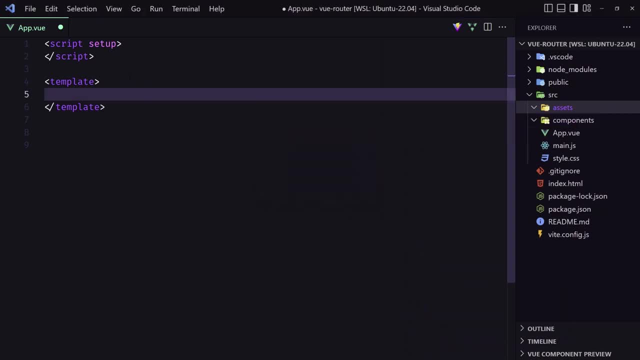 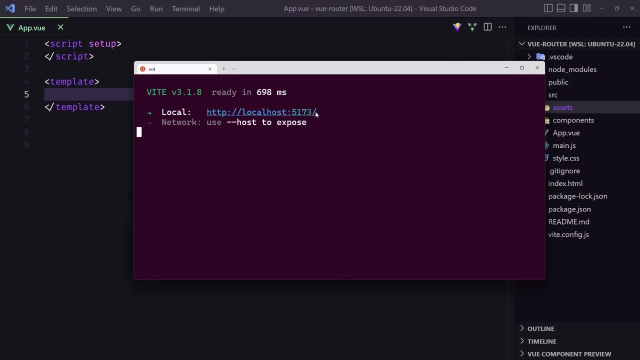 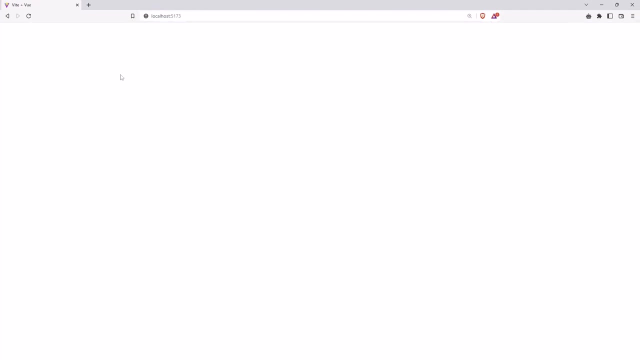 going to delete that. Very good, So I'm going to open the Vue setup and nothing else. Now let's copy this URL and let's open in the browser here. Okay, We have a blank page. We don't have any error Console for now. Very good Now. 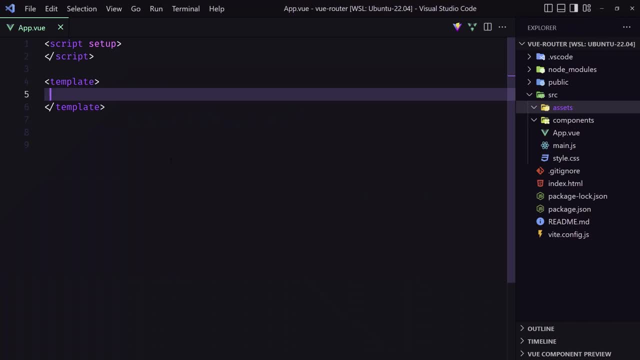 let's go and install the Vue Router. So I'm going to say inhere here in the terminal: npm: install view dash router at 4. for version 4, hit enter. okay, very good. now let's go and create, add the router here in our app and also we need to create some routes. 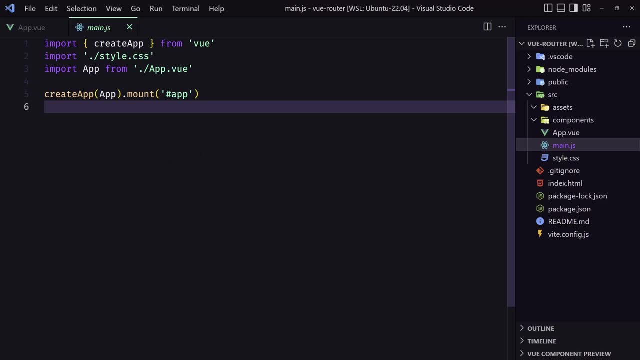 to see how it's going to look. first we need to define the components for our route. for that we are going to: i'm going inside the source directory, i'm going to create a new directory and i'm going to name it views, like in the laravel when we have views. and here i'm going. 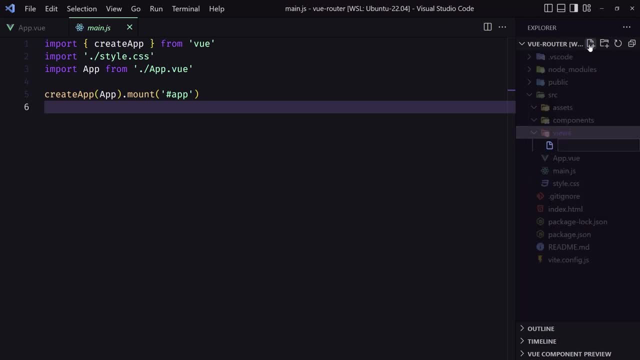 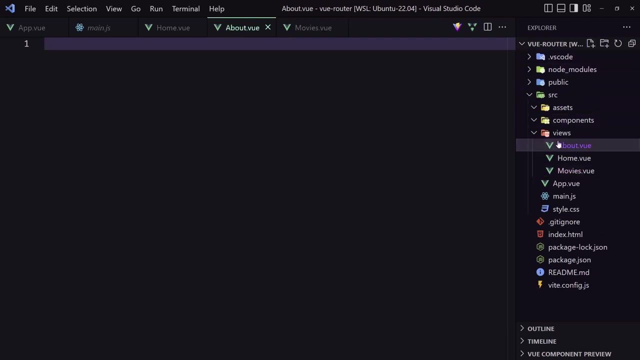 to create two files. so let's say home dot view and the about view, about dot view. and also i'm going to get one more movies dot view, okay. and here i'm going to create a v setup and just say here in the h1: uh, we are in the about, let's say about here. 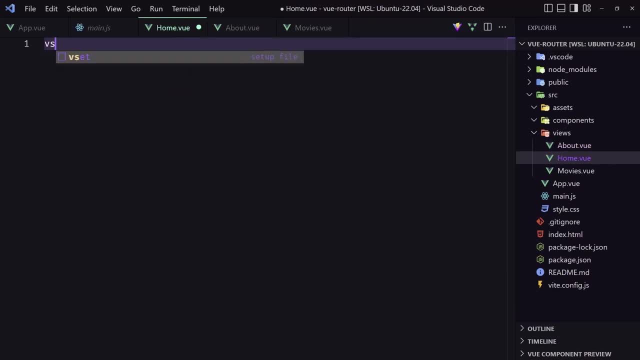 save v setup here and say h1, and here we are in the home. so let's say home here, and the last one is the movies. so let's save this setup and just add one. move this here. very good, save. now let's go in the main js. here we need to import the creator músicajsoncom. it will. 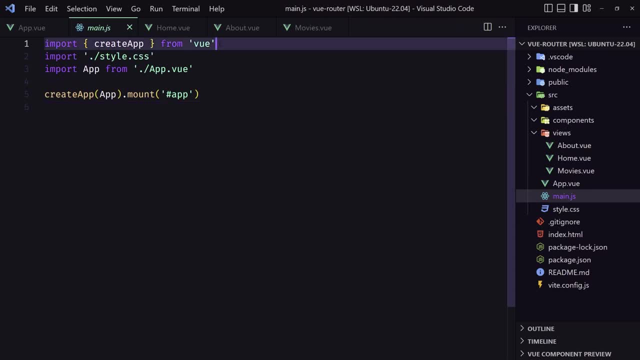 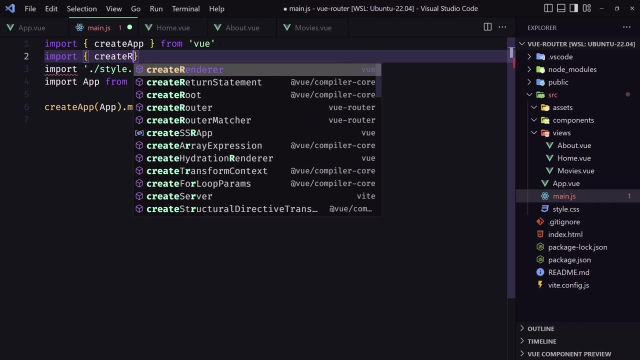 be one from there. now any first title, and then we're going to import the name of the script, so let's say design, and now selectальная, all the rights to the Ramuğ upgrades end router from the view router. so let's say, import the create router from the view router and also 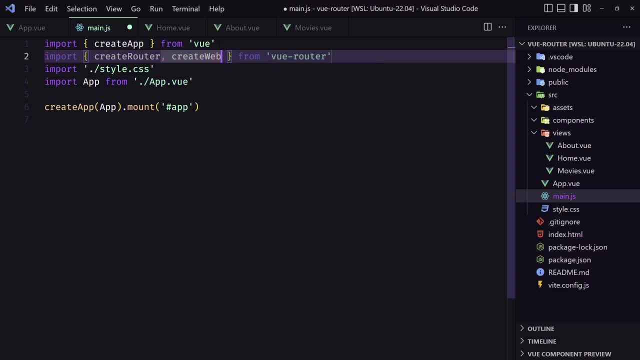 i'm going to import, create web history. i'm going to use web history. if you want, you can use the web hash history. okay, and first i'm going to import the components we need for the routes. so let's import the home component which is inside the, so let's import from. 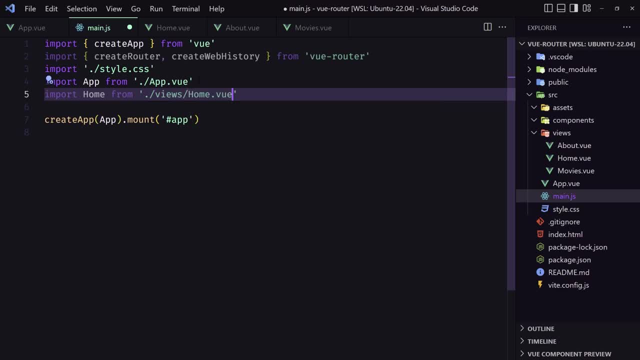 slash views, slash home and change this for the about and this one for the movie. so this is for the movie. this very good. now we have the components we need to define the routes and each route should map to the component we have here. so let's create a constant and say routes, which is going to be able? 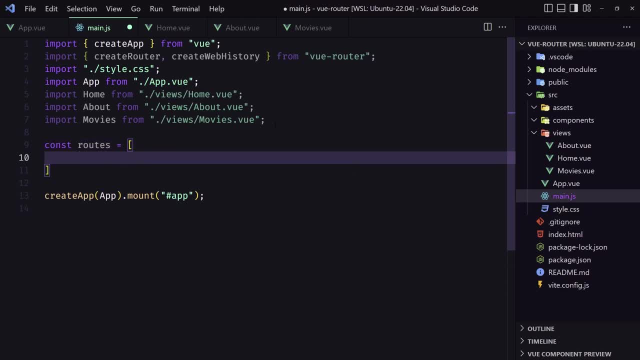 with an array of objects and each object is going to be a road with the path and the component, the load, when we navigate to that path. that's what it's for. so, for example, here an object with path and i'm going to say here a slash. so when we navigate to the home page, i want 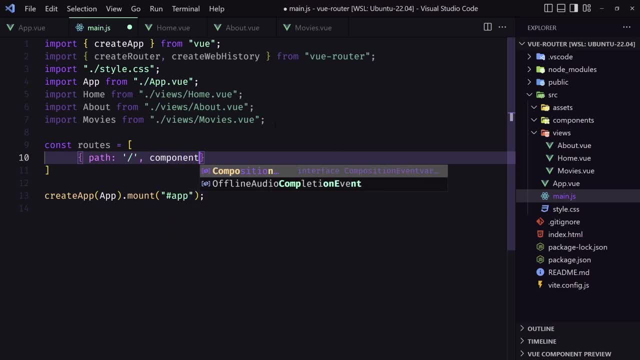 to load the component. so it's a component here, home component. so when we navigate to the slash, we are going to load this component. and now let's copy and paste this. and here i'm going to say: when we navigate to the slash about, i want to render the about component. 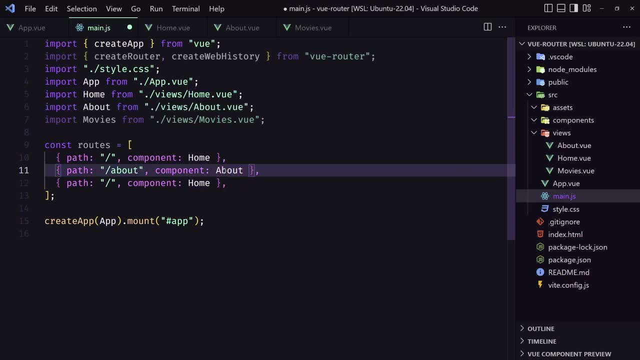 okay. so when we navigate to the slash about is going to load this one. when we navigate here, the home- and now when we navigate to the movies- slash movies- i'm going to load the component. i'm going to say here, load the component, movies, okay, but that is not yet ready, so we need to create. 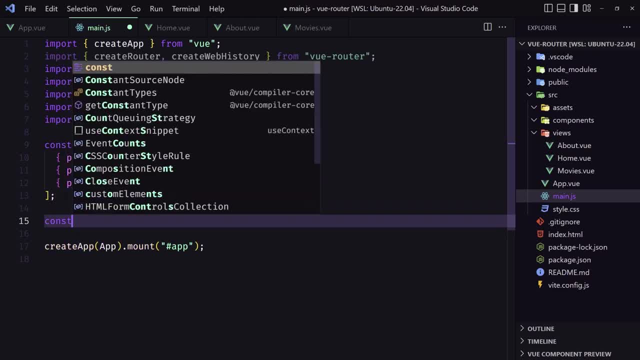 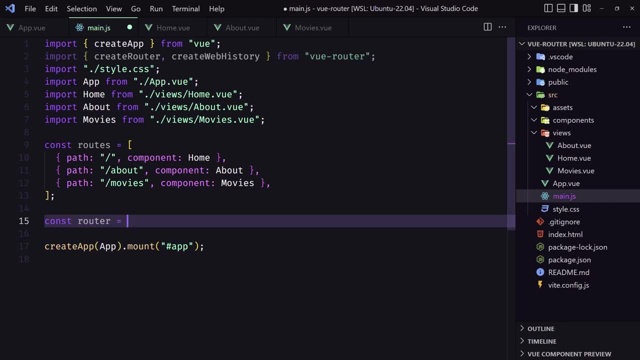 a constant for router, so let's say const router. yeah, like this, which is going to be equal with the create router we have imported from the view router, so let's say create router. okay, here we are going to add an obviously object and i'm going to specify the history to be: 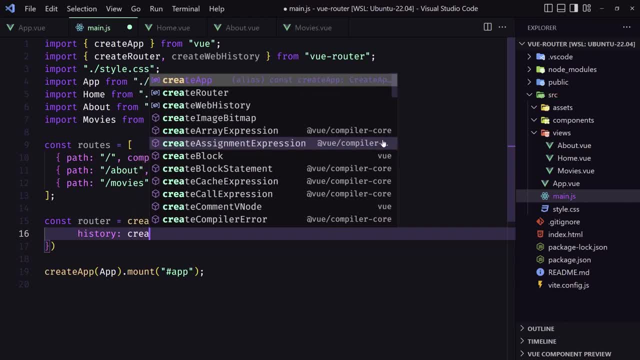 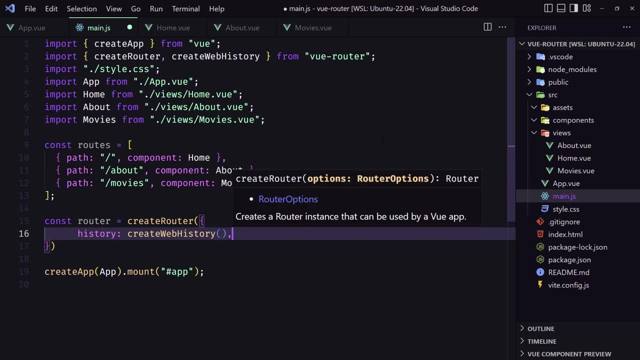 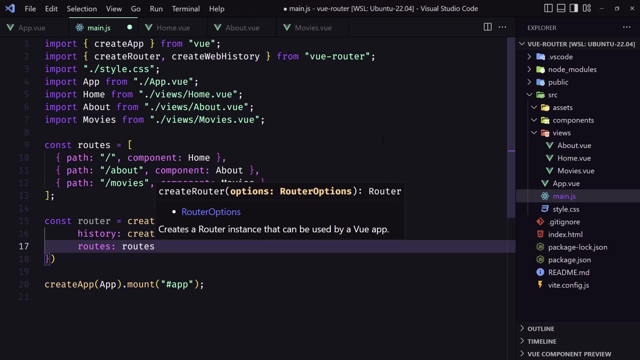 the create web history we have imported from the view router and we need to add routes. here. we can say routes, which is going to be the routes we created, or in javascript six, we just can say like this: and we're going to say the routes we created. 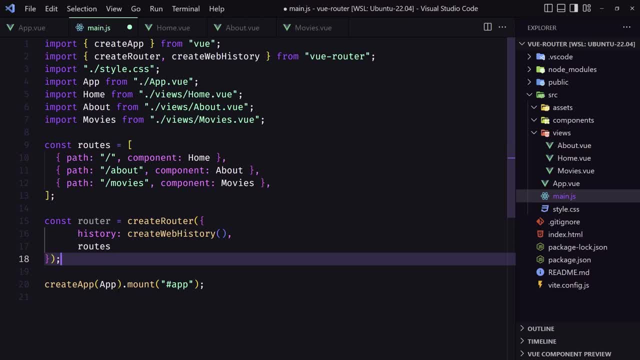 and we're going to say the routes we created, and we're going to say the routes we created, we are okay. and then in the, we are okay. and then in the, we are okay. and then in the: here we can say just use, here we can say just use. 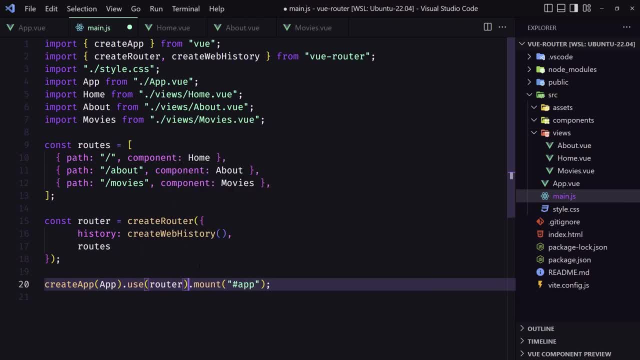 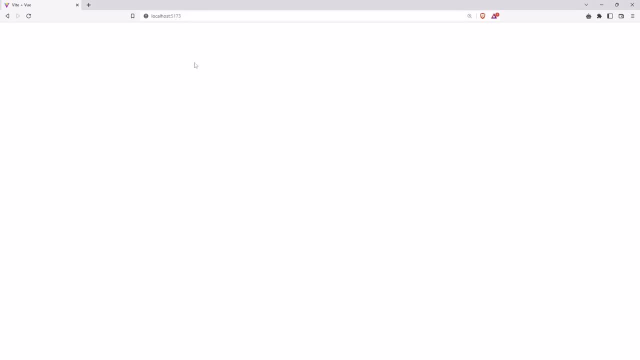 here we can say: just use the router, and let's say: and let's say, and let's say: let's go, let's go, let's go to the project, and if i refresh to the project, and if i refresh to the project, and if i refresh, uh yeah, we don't see anything because we 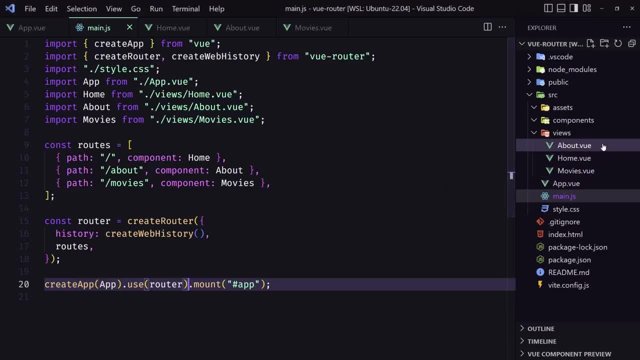 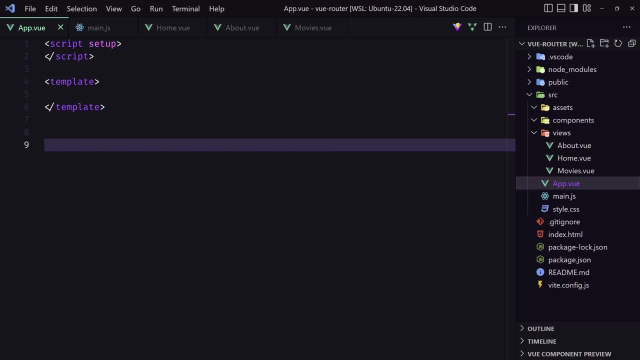 uh, yeah, we don't see anything, because we- uh, yeah, we don't see anything, because we need to go, need to go, need to go inside the inside, the inside, the app view, app view, app view. and here and here and here we need to add the route outlet. 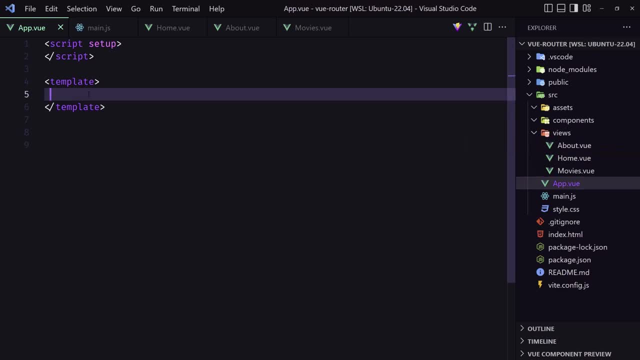 we need to add the route outlet. we need to add the route outlet because right now we have an empty here, because right now we have an empty here, because right now we have an empty here, so let's add, so let's add, so let's add router. 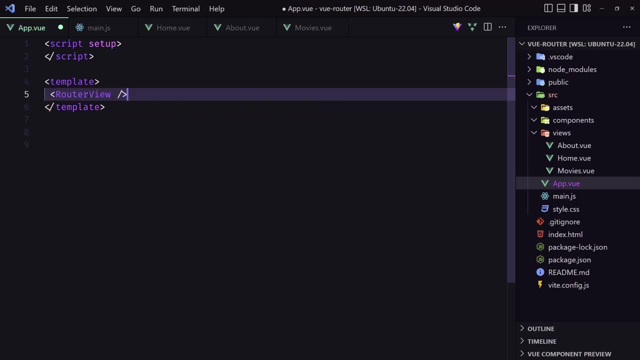 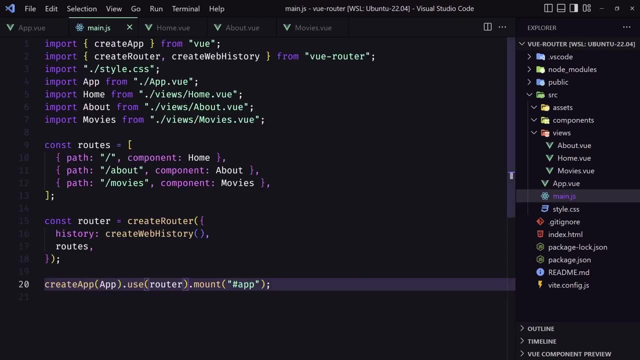 router, router view, view. view like this: and now here and now here and now here: any component matched to the url is going to load inside here. so url is going to load inside here, so url is going to load inside here. so let's say here, let's say here: 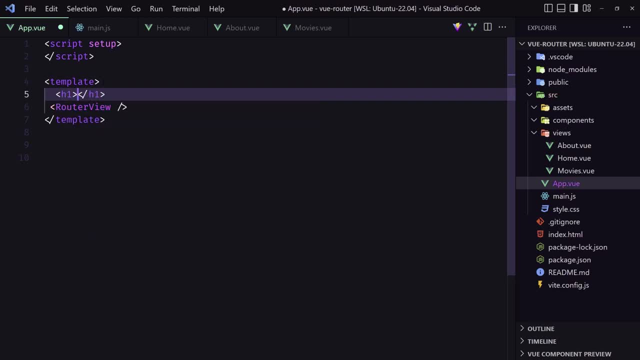 let's say here h1, h1, h1, the, the, the- let's say the header and the components- is going to load and the components is going to load and the components is going to load after the header and the component, so after the header and the component. so 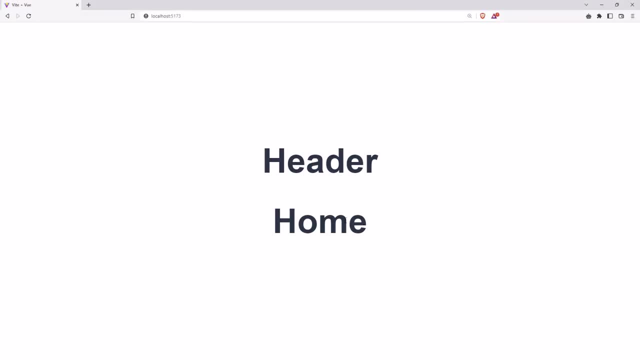 after the header and the component. so let's go here, let's go here, let's go here. and, as you can see, we have header and, and, as you can see, we have header and and, as you can see, we have header and the home, which is the. 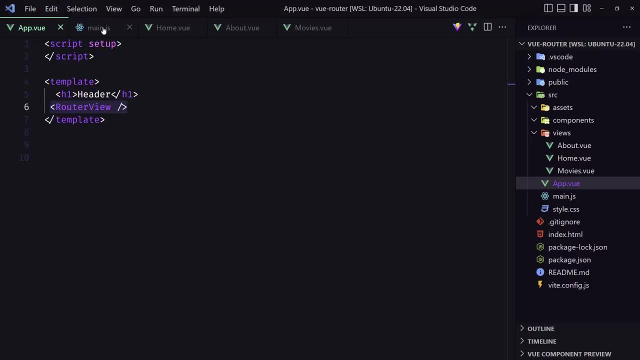 the home, which is the, the home, which is the home component. now, let's navigate home component. now, let's navigate home component. now, let's navigate to the slash, to the slash, to the slash, about, and you can see, so let's copy this about. and you can see, so let's copy this. 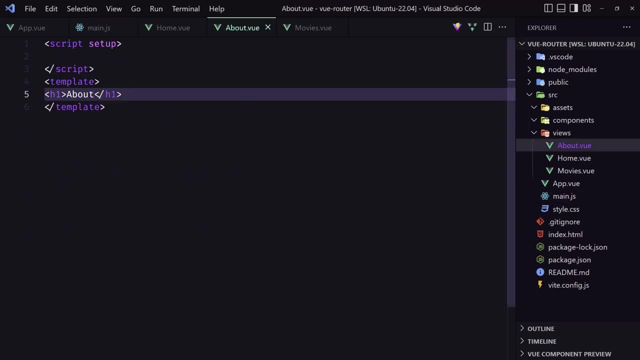 about and you can see. so let's copy this. it's going to render the about. it's going to render the about. it's going to render the about component and the about component has component and the about component has component and the about component has only the h1. 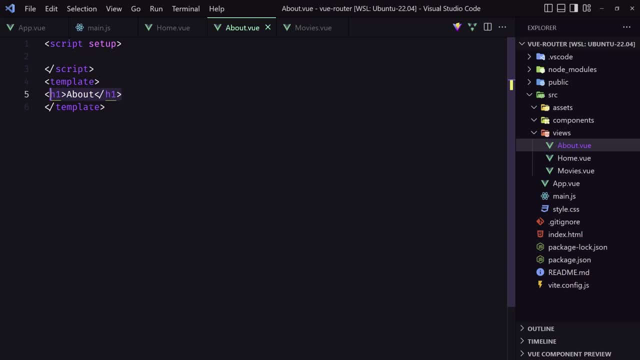 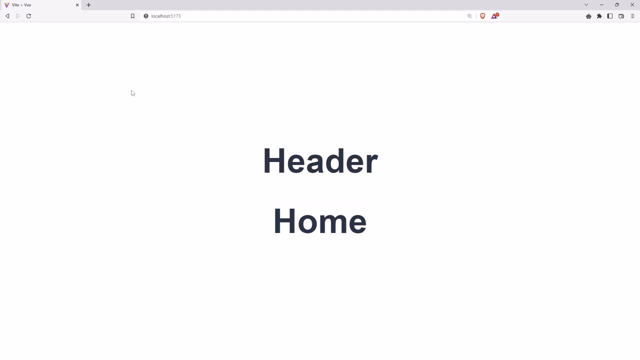 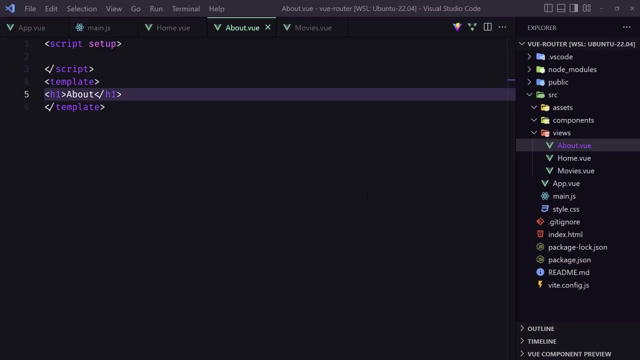 only the h1, only the h1 with about component, with about component, with about component, nothing, okay. so now if i paste that in, okay, so now if i paste that in, okay, so now if i paste that in, we see about here, we see about here, we see about here, because the about component returned this. 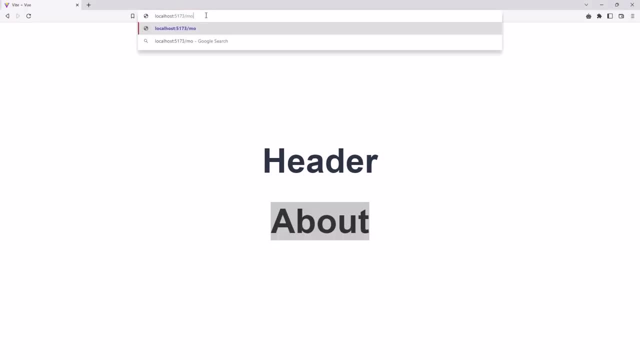 because the about component returned this, because the about component returned this one. and, of course, if we navigate now to one, and of course, if we navigate now to one, and of course, if we navigate now to the movies we see about here, because the about component returned this one, and, of course, if we navigate now to the movies, 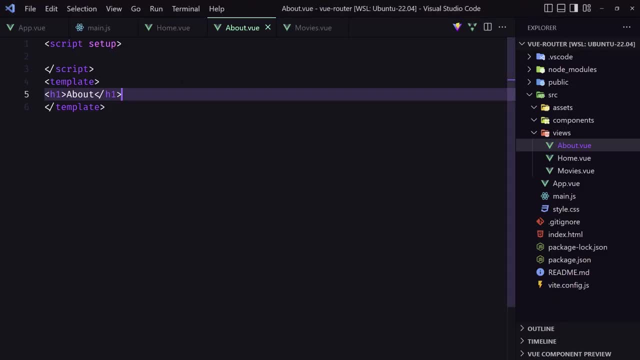 we see about here, because the about component returned this one. and, of course, if we navigate now to the movies we see about here, because the about component returned this one. and, of course, if we navigate now to the movies, we see movies here. we see movies here, we see movies here. okay, friends, that's it, the intro for this. 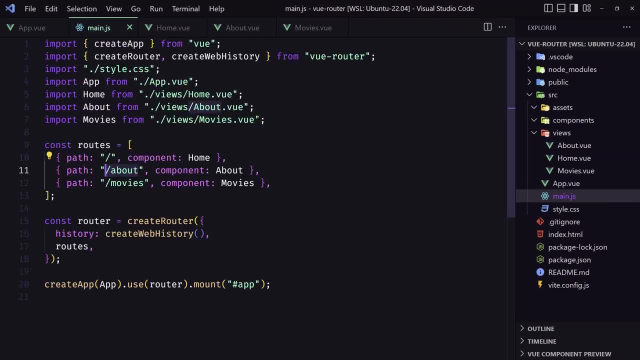 okay, friends, that's it the intro for this. okay, friends, that's it the intro for this. video for the view router. video for the view router. video for the view router. we created the view project, we created the view project. we created the view project, imported the create router and create. 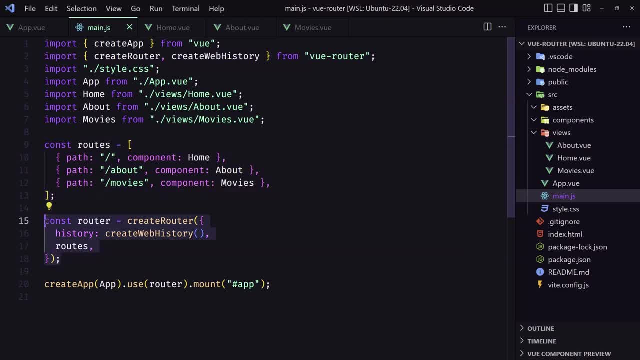 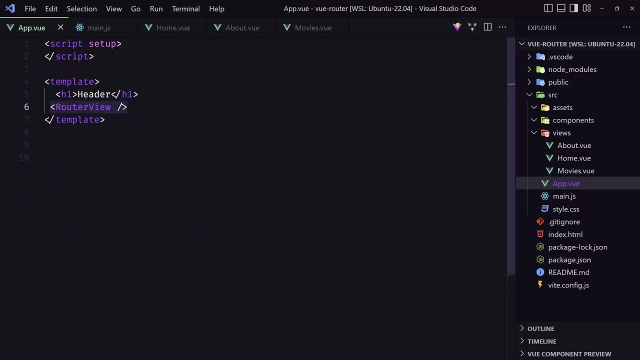 imported the create router and create. imported the create router and create some routes here, some routes here, some routes here, create the router with web history and create the router with web history and create the router with web history and we say use router, we say use router, we say use router and in the app view we added the. 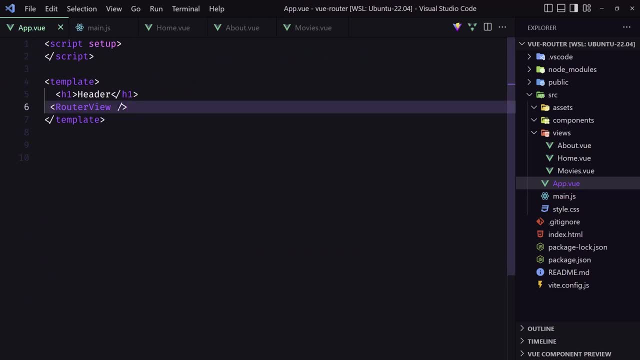 and in the app view we added the. and in the app view we added the router outlet. so any router outlet, so any router outlet. so any of the routes to the route will render of the routes to the route will render of the routes to the route will render in here.